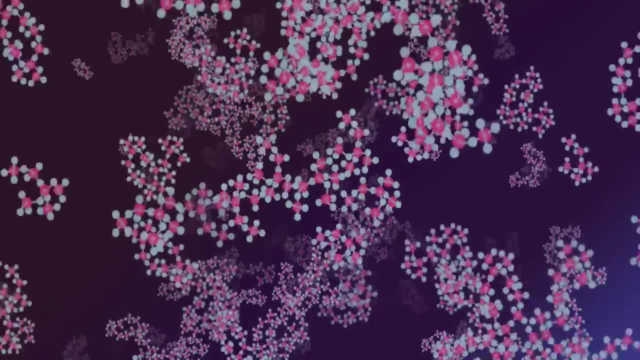 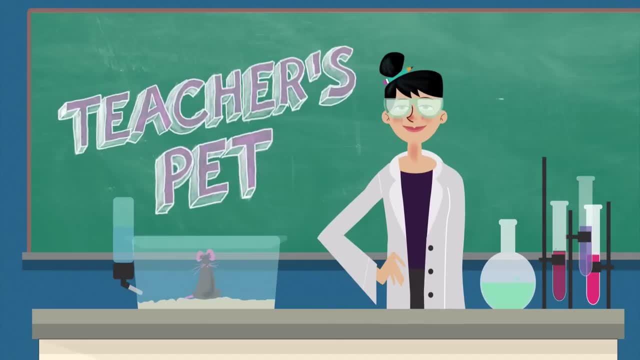 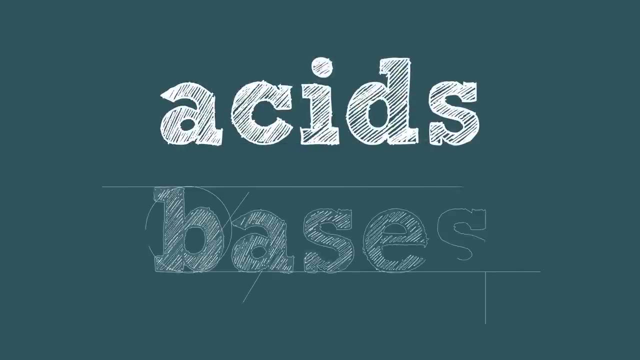 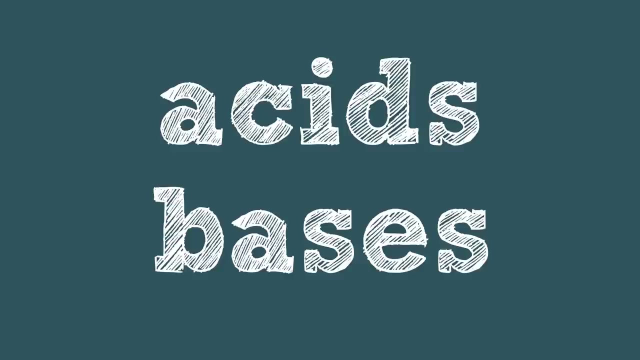 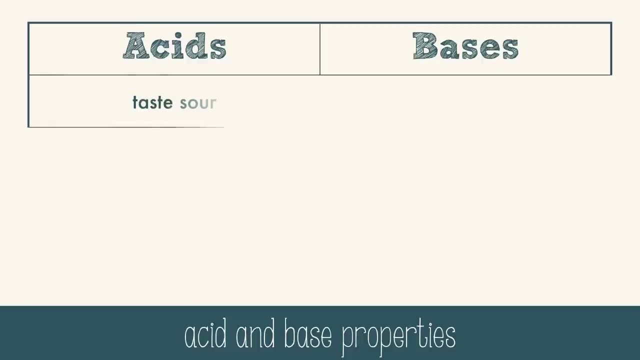 Every day you encounter acids and bases, and you probably ate food with acids in it today and maybe washed the dishes with a base. There are some basic properties that will help you distinguish acids and bases from other chemicals. Acids have a sour or tart taste. Think of lemons or 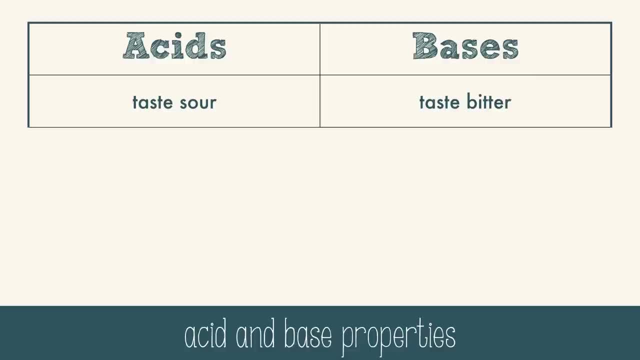 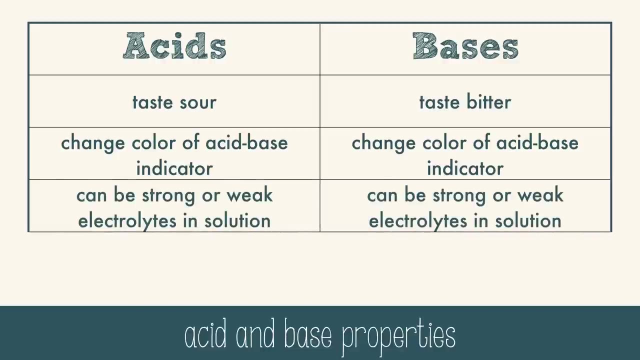 vinegar. That's the taste. Bases taste bitter, which is not a pleasant taste. If you've ever had soap in your mouth, you'll know the taste of a base. Both acids and bases will change color in the presence of an acid-base indicator. They both can be strong or weak electrolytes in 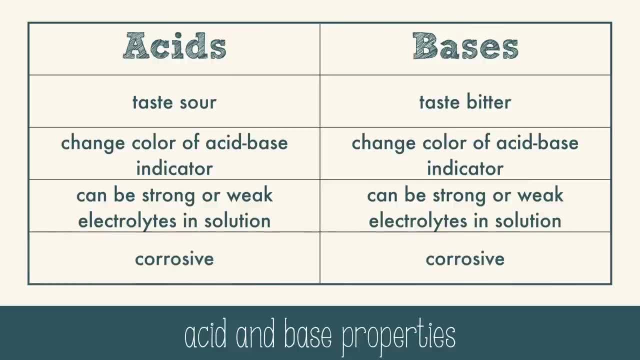 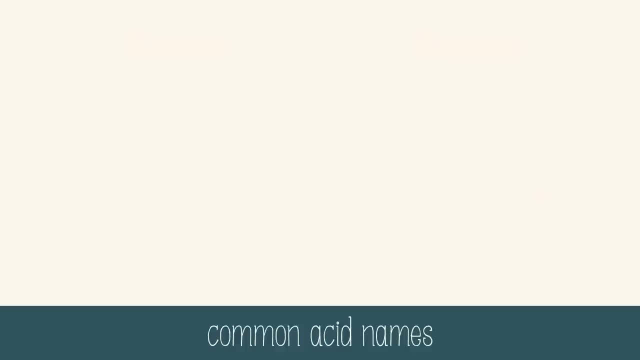 solution and they're both corrosive. Always check the safety information when working with acids and bases to make sure that you protect yourself and your clothing. Acids also have a slightly different naming convention compared to other chemicals. Here are some common acid names that you'll come across in the chemistry lab. 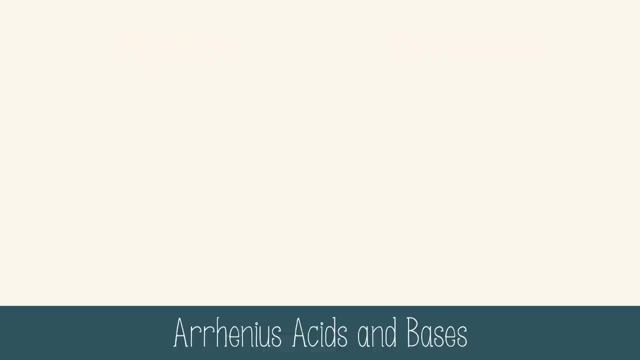 Now, it wasn't until the late 1800s that a scientist was able to propose a theory for what makes an acid an acid and a base a base. That scientist was Fante Arrhenius. He said that acids are hydrogen-containing compounds that ionize to create hydrogen ions or hydronium. 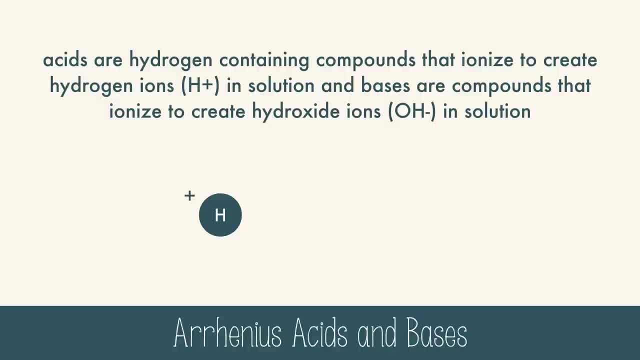 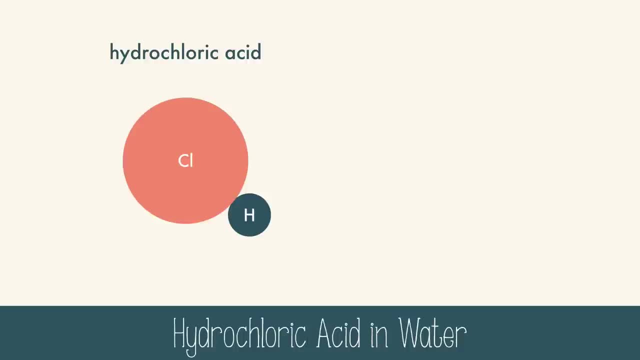 in solution and bases are compounds that ionize to create hydroxide ions in solution. Let's look at an example of this happening. Hydrochloric acid is a hydrogen atom and a chlorine atom covalently bonded In water, the hydrogen abandons the chlorine, leaving its 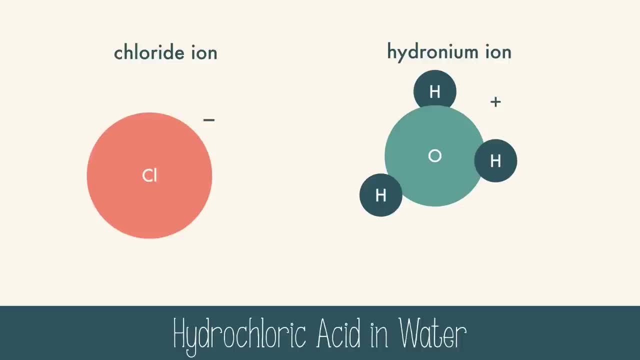 electron behind and then it joins the water molecule to form hydronium ion. Because hydrogen can be removed as an ion, hydrochloric acid can be removed as an ion and hydrochloric acid can be removed as an ion. Hydrochloric acid releases one hydrogen, so it's called monoprotic. Some 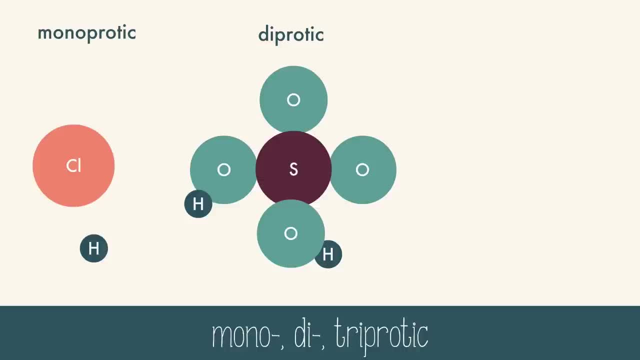 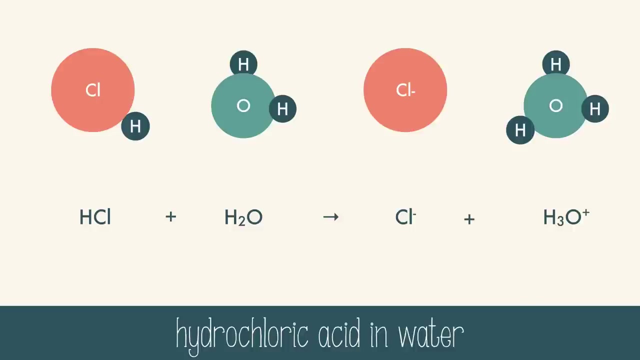 acids have multiple hydrogen atoms that will ionize and could be diprotic if they release two hydrogen ions, like sulfuric acid, or triprotic if they release three hydrogen ions, like phosphoric acid. Let's look again at hydrochloric acid in water. Hydrochloric acid. 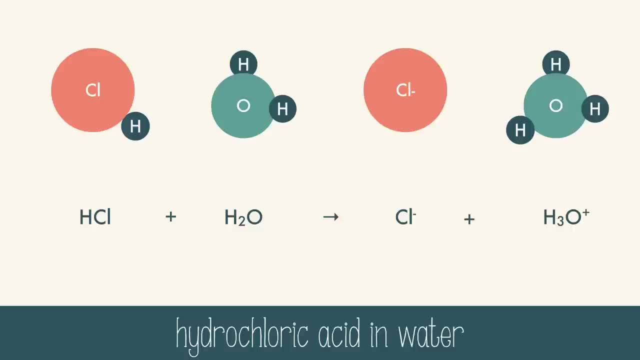 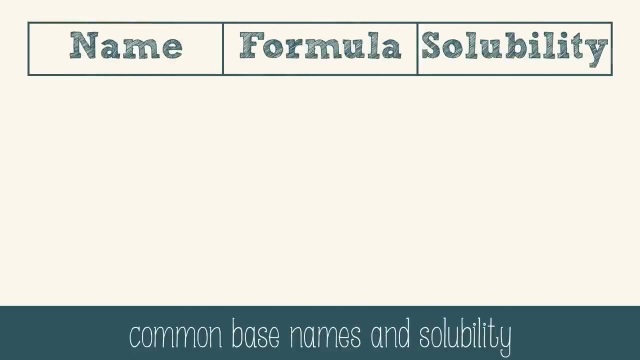 is an Arrhenius acid because it creates a hydrogen ion. The hydrogen ion immediately attached itself to water to form hydronium H3O+, which is the aqueous form of hydrogen ion. Arrhenius bases produce hydroxide, so it's no surprise that all of these bases have hydroxide. 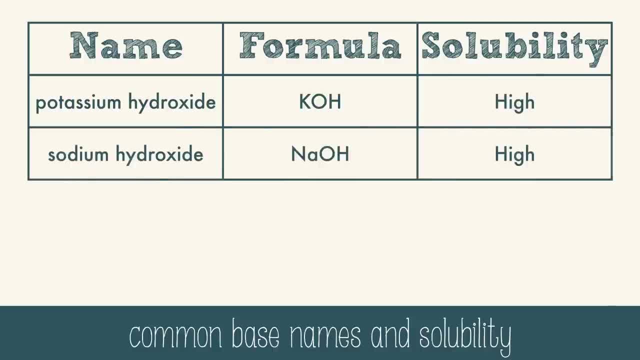 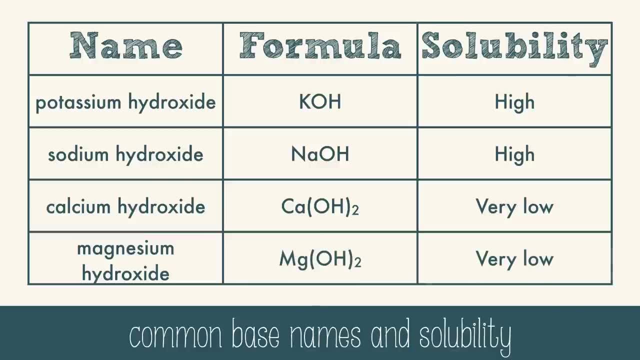 in their names, Potassium hydroxide and sodium hydroxide are strong bases and are very soluble. Calcium hydroxide and magnesium hydroxide are also strong bases, but they don't dissolve easily in water, which makes the solution very diluted. 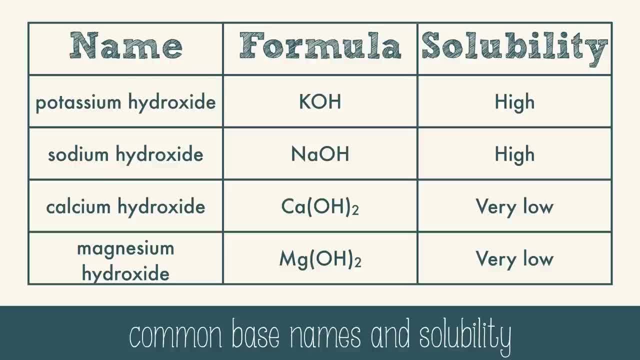 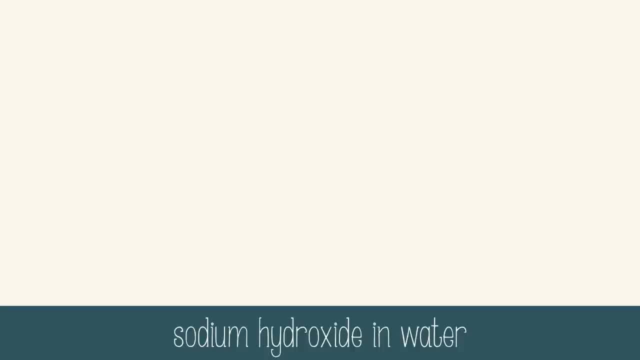 Now let's look at a base in water. We'll use sodium hydroxide. Sodium hydroxide is a sodium attached to an oxygen and hydrogen, which is the hydroxide ion, And when it breaks apart in water, you'll get a sodium ion and a hydroxide ion. That hydroxide ion is what makes this a base, Because the sodium hydroxide was able to make that. it's an Arrhenius base. 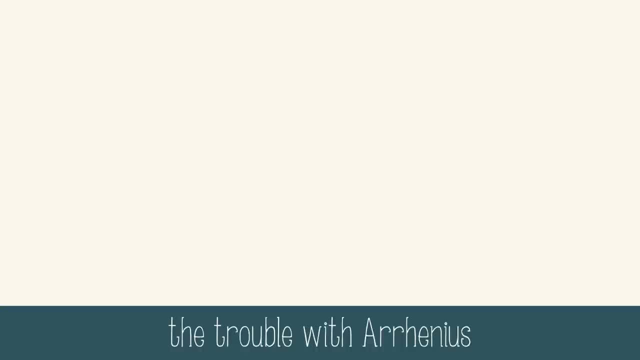 The Arrhenius definition, it turns out, is too confining for all acids and bases. For example, ammonia is basic, but there's no hydroxide on ammonia. In the presence of water, however, it will react to produce hydroxide from the water molecule. So there is another. 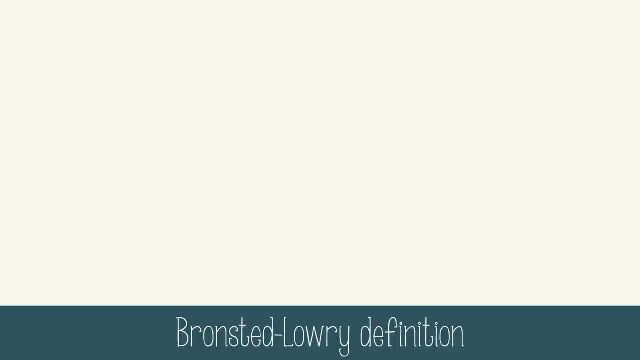 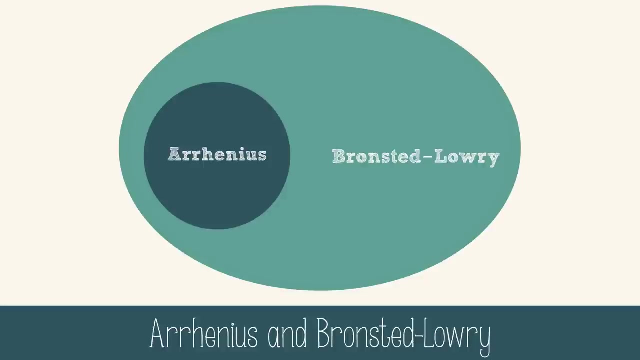 way to define acids and bases. The Bronsted-Lowry definition is that acids are hydrogen ion donors and bases are hydrogen ion acceptors. It's a broader definition. acids and bases are also Bronsted-Lowry acids and bases, but not all Bronsted-Lowry acids and bases. 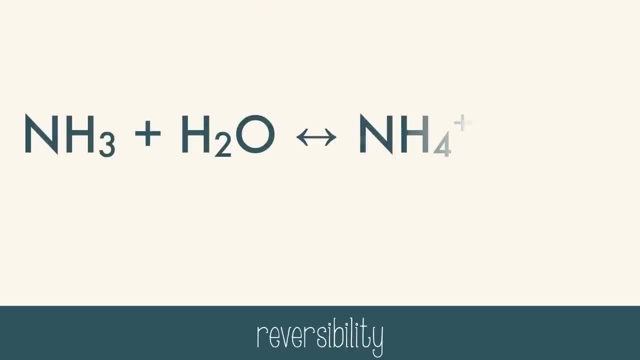 are Arrhenius. When you look at an acid-base reaction, you'll notice that a double arrow is often used. This implies that the reaction is actually reversible. It can occur in both directions. In this reaction, the ammonia is the base because it's the hydrogen acceptor By default. 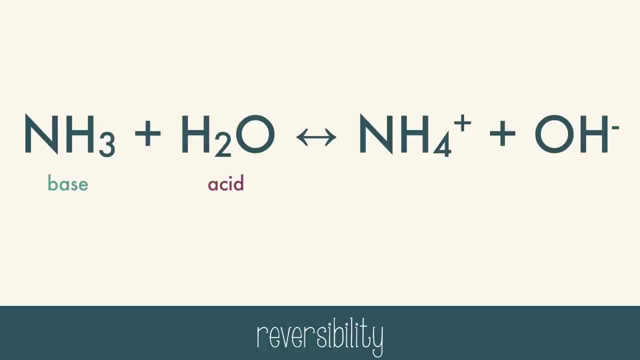 then the water is acting as an acid because it will be the hydrogen donor. But when we look at the other side of the equation, we could imagine it going to the opposite direction, where ammonium ion would donate the proton and hydroxide would accept. We call these the conjugate acid and the